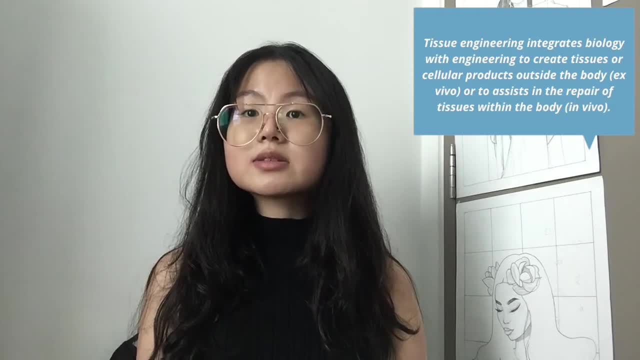 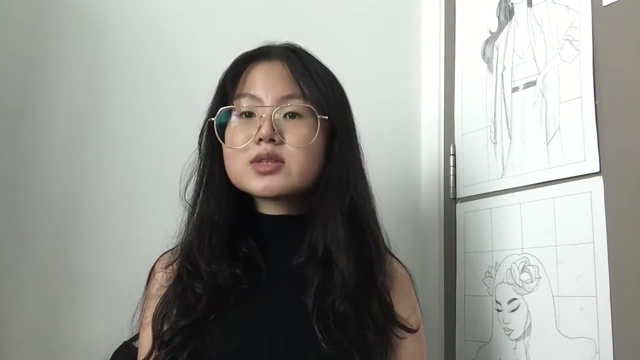 with engineering to create tissues or cellular products outside of the body ex vivo or to assist in the repair of tissues within the body in vivo. This requires understanding of various biological fields, ranging from cell and molecular biology to extracellular matrix chemistry and compounds. It also 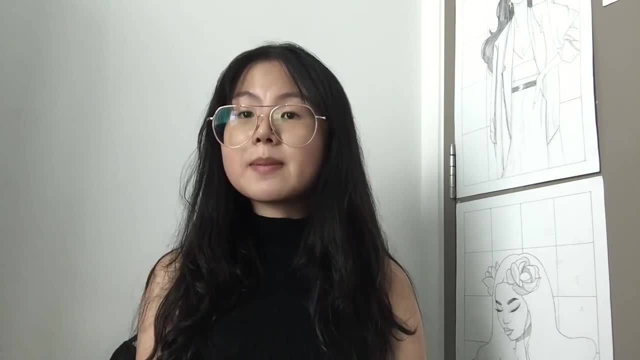 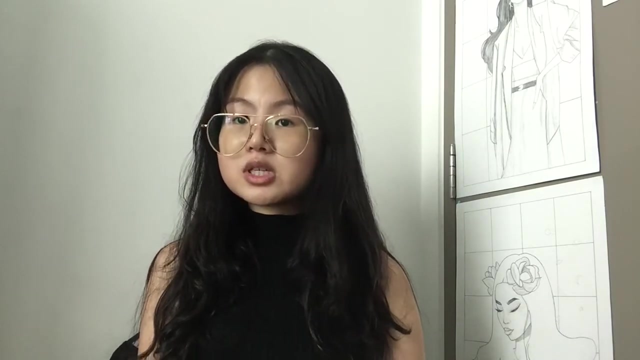 requires knowledge of engineering fields such as biochemical and mechanical engineering. This has also contributed to the field of regenerative medicine, which is similar to tissue engineering but focuses more on the strategies that use the body's natural regeneration mechanisms to repair damaged tissues. Human tissues have been studied for thousands of years In ancient Egypt. 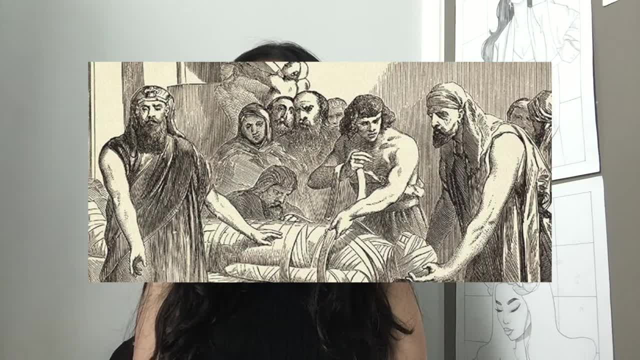 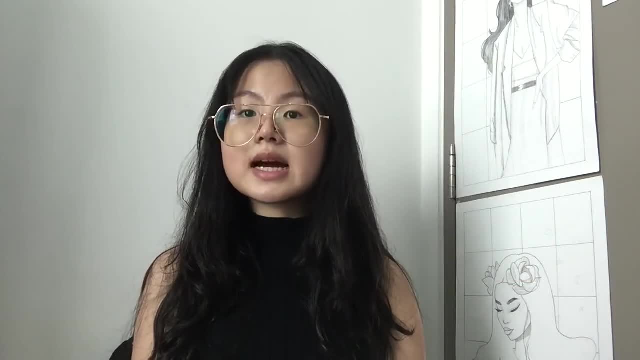 physicians studied corpses of living humans in order to understand how to treat wounds by grafting skin from corpses to living humans. Moreover, between 1069 and 664 BC, skin grafts and transplants were discovered on mummies and corpses of women. 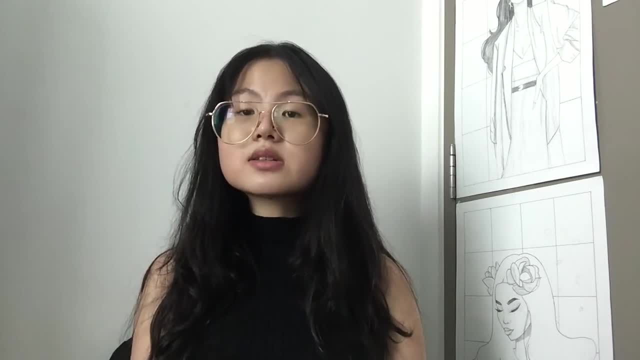 In 1931, signs of dental implants were discovered in a jaw belonging to a Mayan woman which dated all the way back to 600 AD. This is perhaps the earliest evidence of tissue engineering being used in America. The main goals of these fields involve the injection or engraftment of cells or cellular. 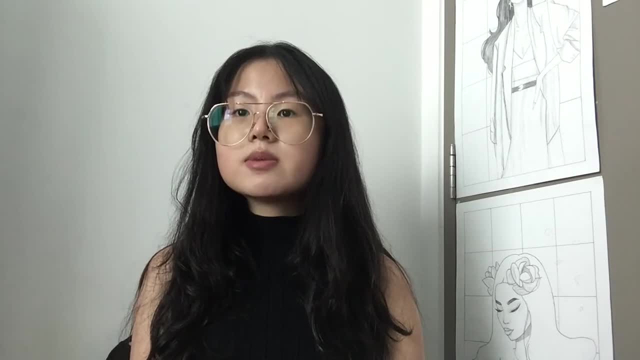 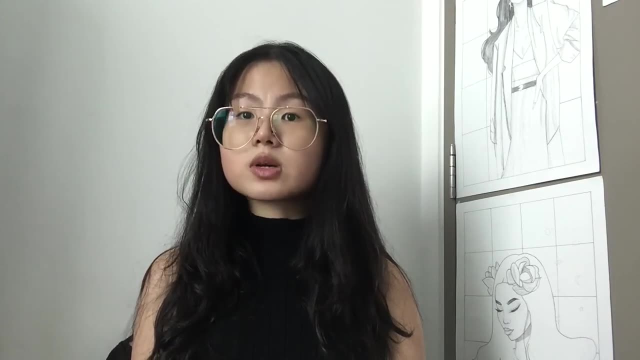 suspension, as well as using tissue ex vivo to be used as grafts or extracorporeal organs, which helps assist or supplement ailing in vivo organs. These are examples of cell therapies for the repair of damaged tissue. Moreover, tissue engineering strategies have been helping with the 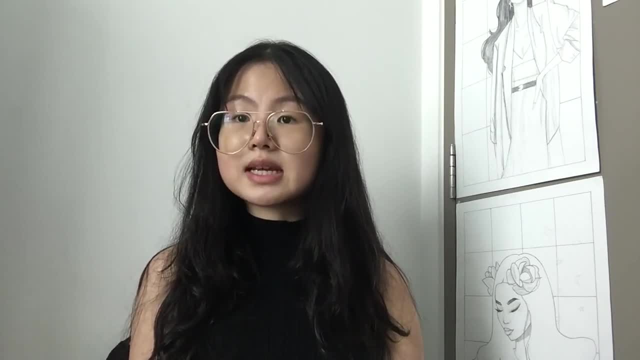 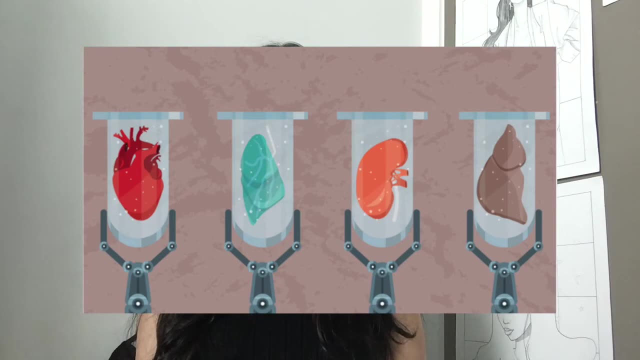 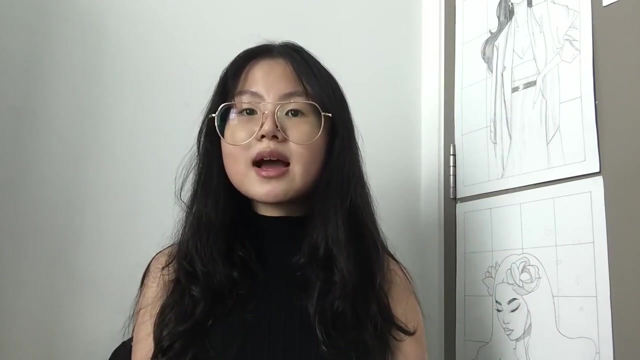 development of improved in vitro diagnostic and screening techniques, as well as creating improved tissue models to study diseases. Another goal of tissue engineering is to create artificial organs through biomaterials for patients that need organ transplants. Currently, researchers have grown solid jaw bones and tracheas. 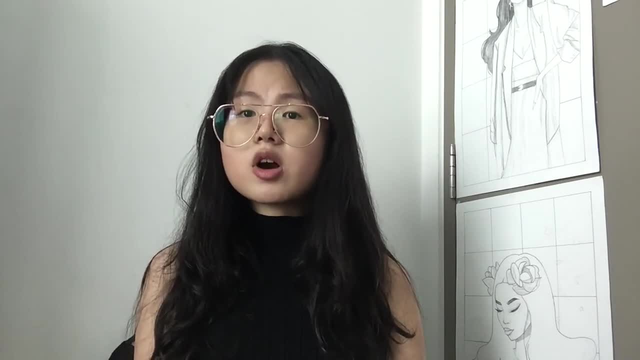 The most common organ transplants are the human stem cells. Not only that, several artificial urinary bladders have been grown in laboratories and have been transplanted successfully into human patients. Bio artificial organs are also currently in development and use both synthetic and biological components, For example. 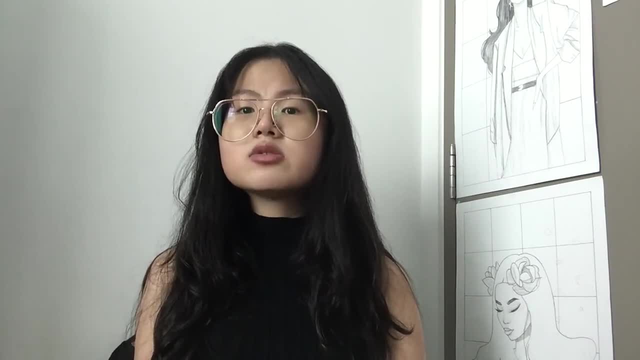 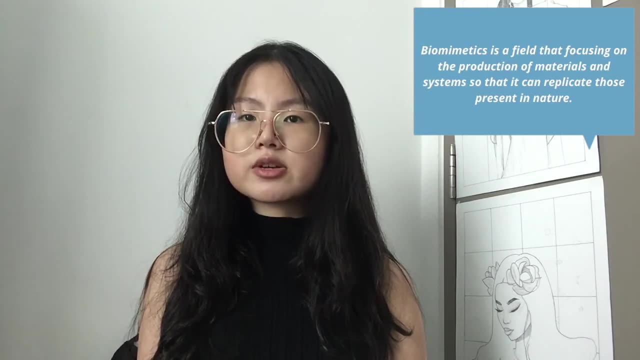 hepatic assist devices have been developed and uses liver cells within an artificial bioreactor construct. Biomimetics is a field that focuses on the production of materials and systems. Biomimetics is a field that focuses on the production of materials and systems. Biomimetics is a field that focuses on the production of materials and systems.